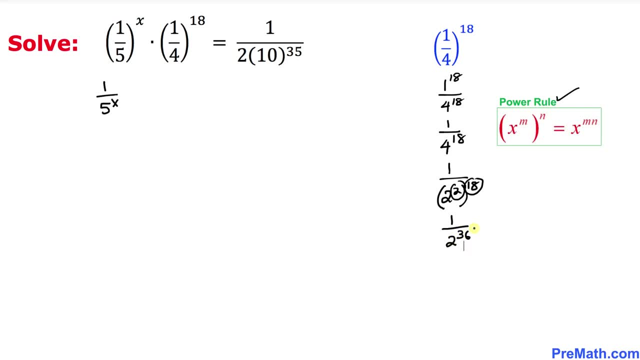 2, power 36. so therefore i can write this one over here: 1 over 2, power 36. and now, on the right hand side, let's focus on this part: 10, power 35 in the denominator, and here i have copied down: let's go ahead and simplify this thing: inside this parentheses: 10. 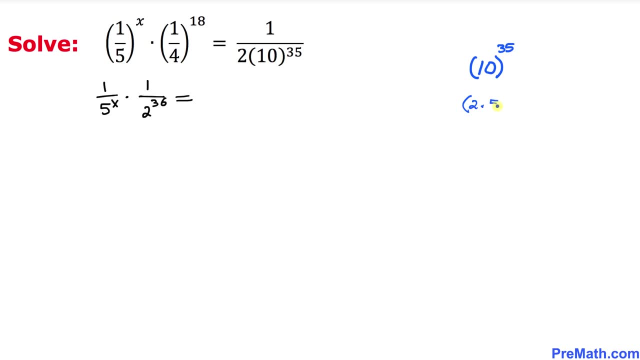 could be written as 2 times 5 and then power 35 and this could be written as a 2 power 35 times 5, power 35. so thus on the right hand side this fraction i can write as 1 divided by 2 times. 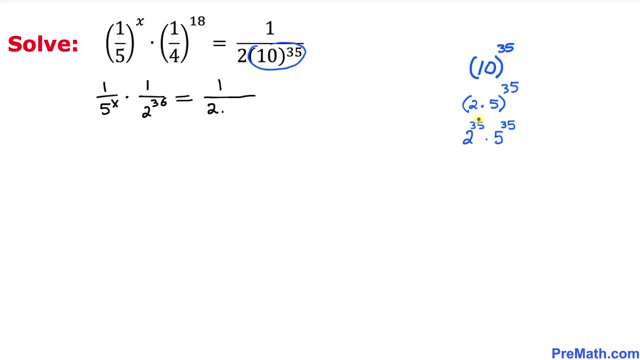 now i'm going to replace this part by this simplified form so i can write: 2 power 35 times 5 power 35. so let's focus on the left hand side of this equation. so this could be written as: 1 divided by 5 power x times 2 power 36. 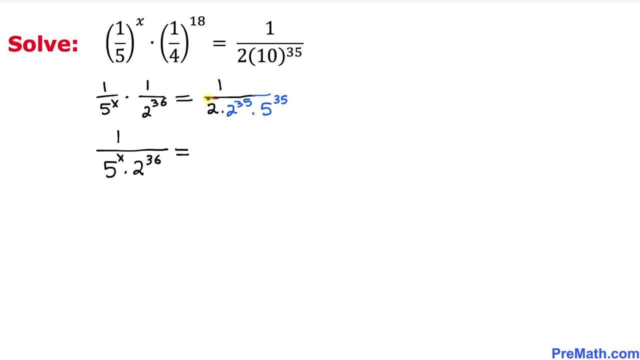 equals 2, and now let's focus on this part. 2 times 2 power 35. and here i have copied down 2 times 2 power 35. 2 could be written as 2 power 1. now let's go ahead and apply this product. 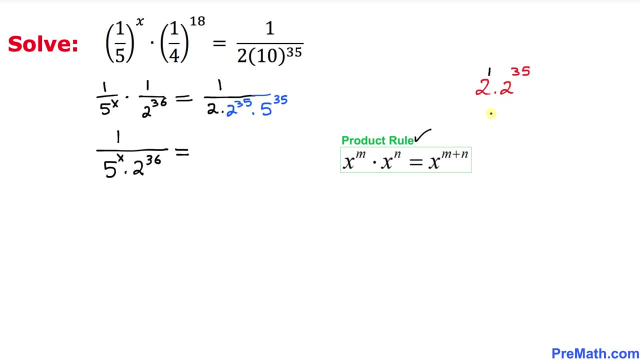 rule. according to this rule, when we multiply these ones, we are going to add their exponent, so this could be written as: 2 power 1 plus 35 is same as 2 power 36. so therefore, on the right hand side, this fraction could be written as 1 divided by 2 power 36 times 5 power 35. and in this next, 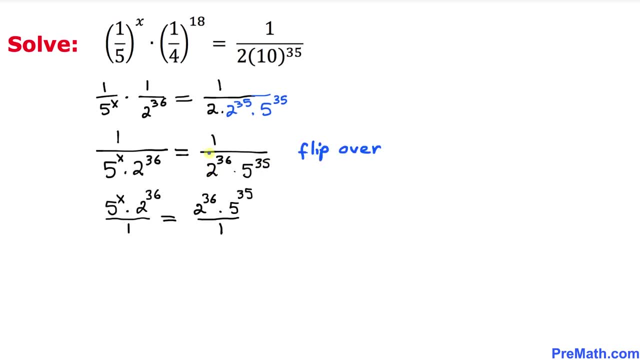 step, we flipped over both sides of this equations, so the numerator becomes denominator and denominator becomes numerator, as you can see over here and now, in this next step, we are going to remove this 2 power 36 from both side. so let me go ahead and divide both side by 2 power 36 on this side and 2 power 36 on this side. 2 power.